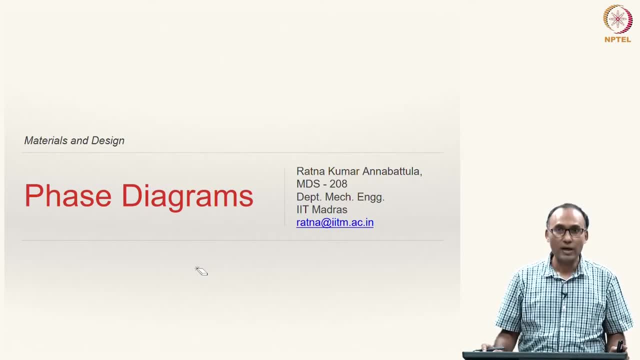 will come in the next course on design of machine elements And once having done that, when, if you remember, in the very beginning, we have discussed the concept of PSPP diagram. So performance structure- sorry, processing structure- and performance and product right. 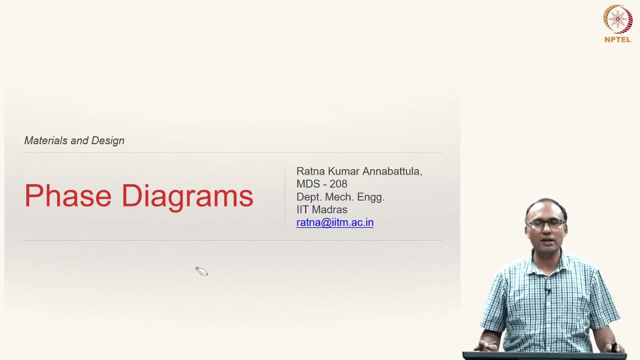 So in that PSPP diagram, the first one is processing, which will give us certain crystal structure. So in this module we will see how this processing helps us in obtaining the structure of our interest. So phase diagrams is a module that actually gives us more understanding about the development. 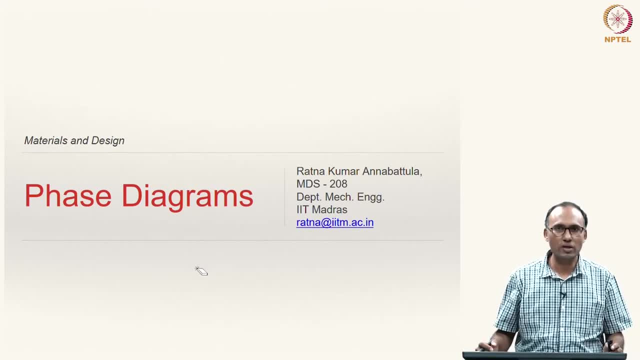 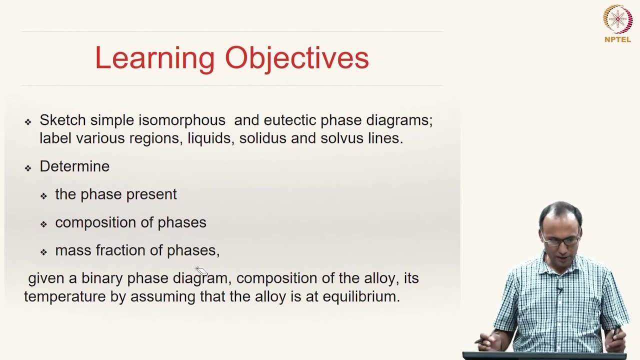 of the structure of a solid material when it is cooled from the liquid state. all right, So the learning objectives of this model are so one. by the end of this module, we should be able to sketch simple, isomorphous and eutectic phase diagrams, And we should 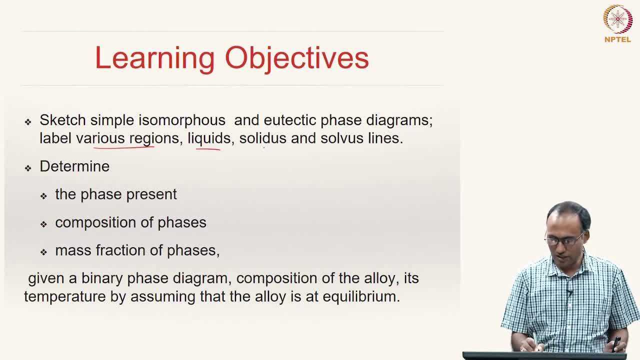 be able to label various regions, such as liquidus, solidus, solvus lines, single phase regions and so on, And in various regions. in this phase diagram, we should be able to determine the phases present and their compositions and the mass fractions or weight fractions of those faces. 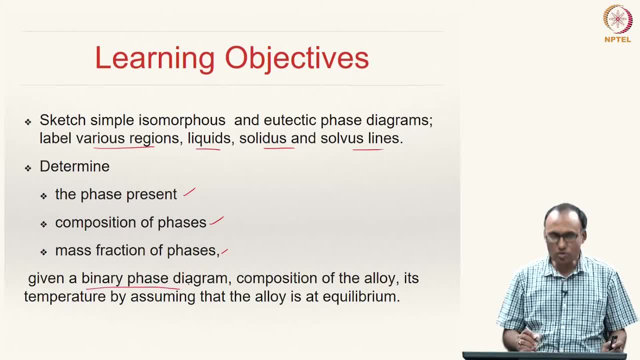 that are present in a binary phase diagram, And in this course, we will be only focusing on binary phase diagrams. What do we mean by binary phase diagram? we will discuss in a moment. And so, given a binary phase diagram and the composition of the alloy and its temperature, 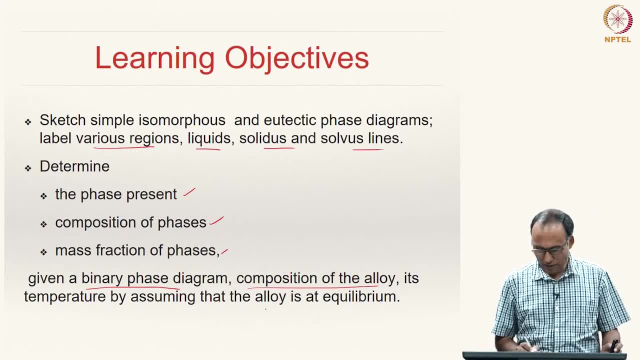 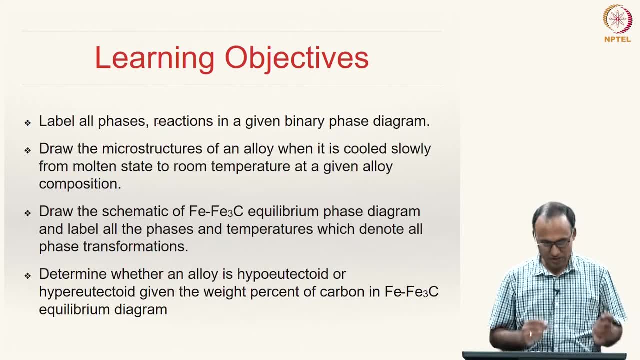 and all this we will do with the assumption that the alloy is at equilibrium right, And then we should also be able to label all the phases in a given phase diagram and the reactions that are present in the that the liquid or solid goes through when it is cooled down. 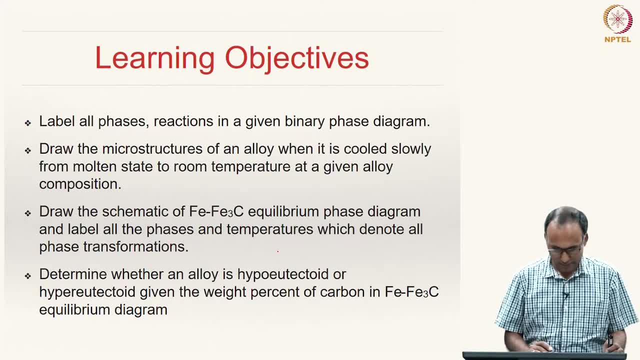 from the high temperature to room temperature or low temperature. And then we should also be able to draw different kinds of microstructures. So when we say draw the microstructure, we actually mean the schematic representation of the microstructure of an alloy when it is cooled slowly from molten state to room temperature for a given 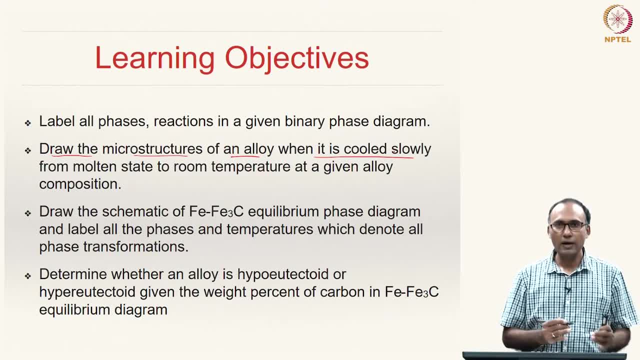 alloy composition And then, once we understand this aspect of understanding different, identifying different phases, calculating the microstructure- we will provide some weight fractions of each and every phase, and so on. We will focus spend a little time on understanding a specific phase diagram of interest to primarily for. 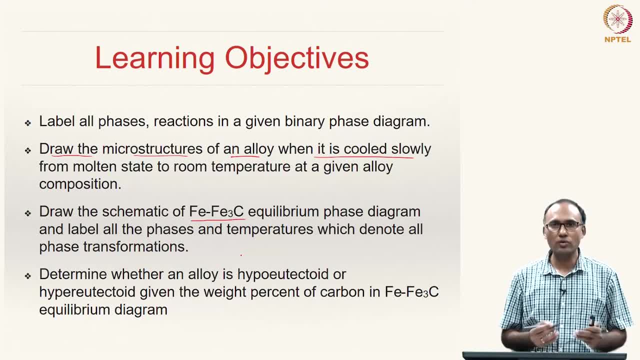 engineers is iron-iron carbon equilibrium phase diagram. So iron carbon phase diagram is of extreme importance, particularly for mechanical engineers, because most of the components or machine components that we work with are made of steel, which is an alloy of iron and carbon. So, and hence we will spend a significant amount of time in this, of this course understanding 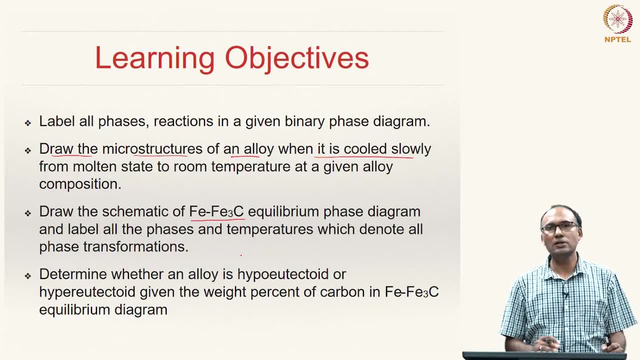 the iron-iron carbide equilibrium phase diagram and the and the discussion thereafter right. And we should also be able to determine, given a composition, whether an alloy is hypo-eutectoid or hyper-eutectoid, given the weight weight per weight fraction or the composition of. 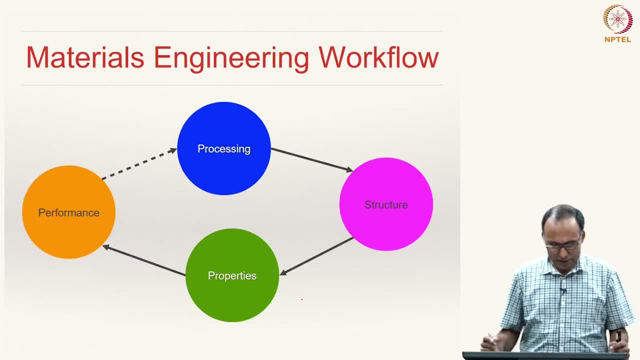 the alloy. all right, So this is our materials engineering workflow, where we have discussed the PSPP diagram: processing, structure, property and performance. However, when we have drawn this diagram in the beginning, we did not have this dashed line. this is something that I have drawn to actually keep. try to make some sense out of the diagram. 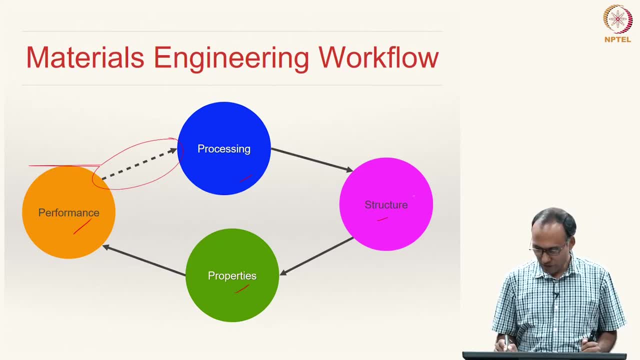 This processing. So as we, as we have discussed, we have actually started here. our journey of this course started understanding the structure. from there we understood the mechanical properties, which strongly, or a function of the underlying microstructure on underlying structure of the solid, And having understood the properties, we have discussed the failure theories and 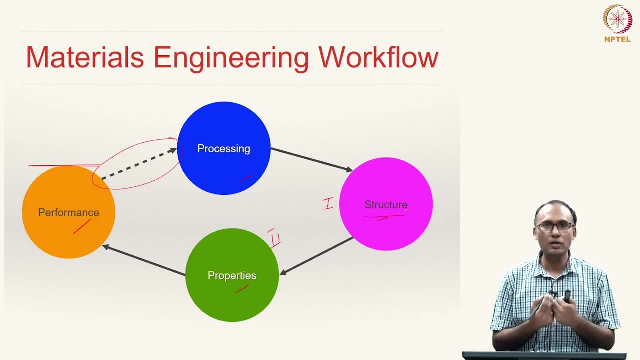 then, based on That, for under given loading condition, what is the factor of safety or whether the component will withstand the loads that are applied. In other words, we are actually- we were actually- trying to understand the performance characteristics of the component, given a particular material being used as the basis for making the component. So we have also in some sense looked at the 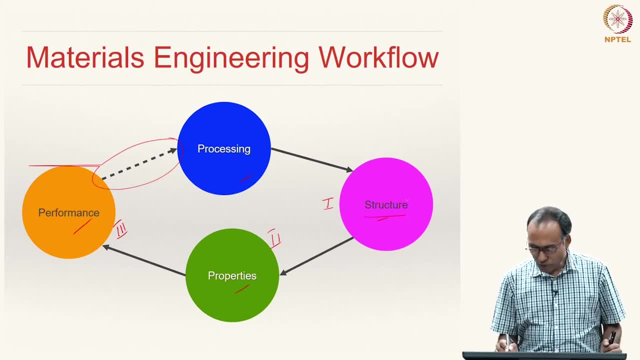 performance. So we know that a particular structure of a material is obtained by taking a different, taking a specific processing route. So the processing is the key which will give us certain structure right, And that structure in turn gives certain properties that those properties are responsible for the performance. Now 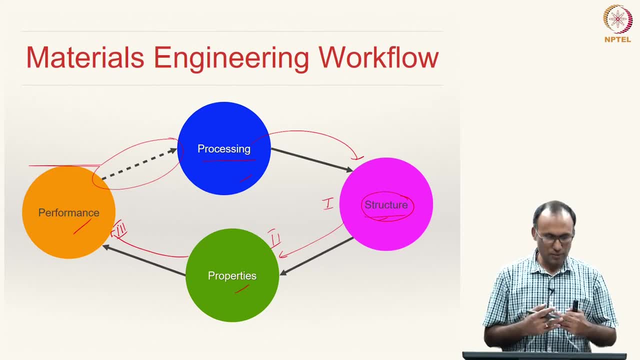 once we look at the performance and then let us say the performance of the component is not of to mark and we need to enhance the performance. And then we have to understand the performance of the components, of the components, for these components here. So this: here are the sake 1 and the. 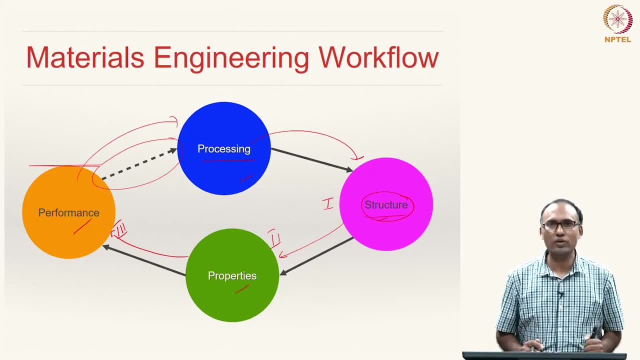 2 and so further. B- China, It is a, B, B C, B, C, B C. So rather look at this module: in case of B is found, like asence, Normally at B. it is not necessarily 보опчи. 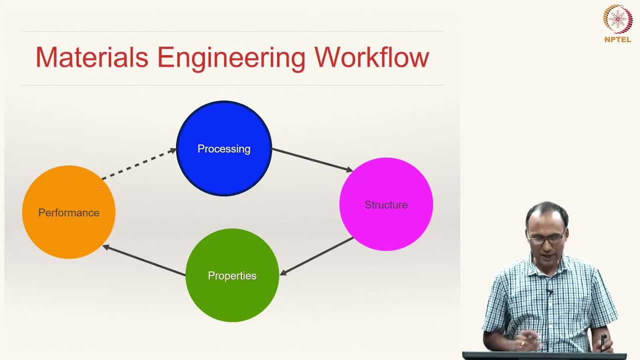 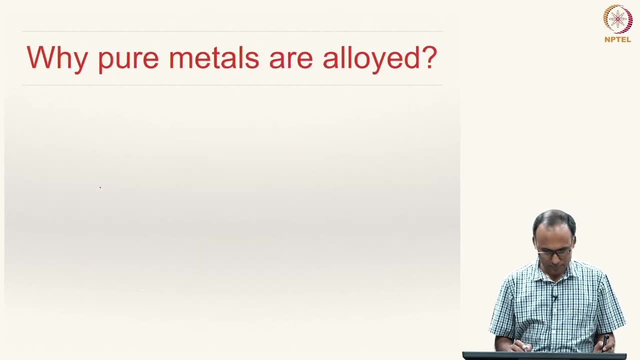 It was. It is not necessarily 보опчи, But if you극 actually discussing the phase diagrams module, primarily discusses the processing part of the PSPP diagram. So the question that we need to ask ourselves is the following: why pure metals are alloyed? Because most of the materials that we use. 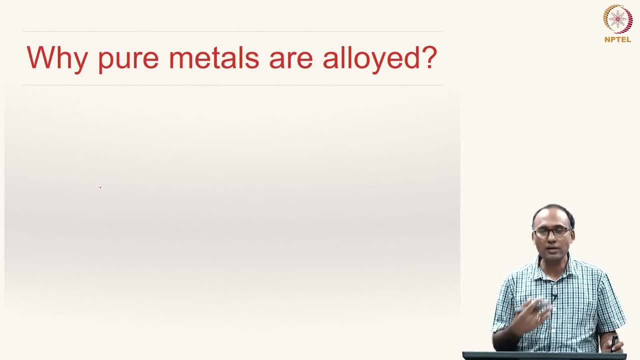 on our daily life are not pure metals. they are almost all the time, or many times they are alloys. So the question is why pure metals are alloyed. So when you take a pure metal, the pure metal strength, for instance, yield, strength and tensile- 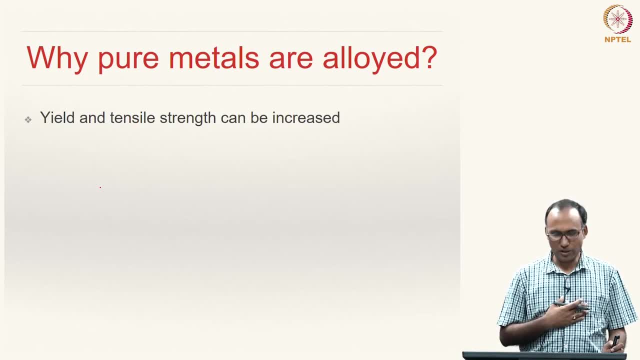 strength from the mechanical properties perspective can be enhanced by alloying it. We can increase the hardness of a pure metal by adding additional components or by alloying it, And we can also change or increase the melting point of the solvent by alloying it, So it is a solvent if you are talking about. 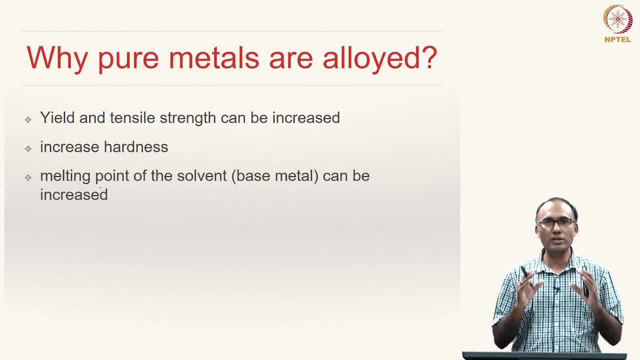 a, an alloy. basically you have two more than one kind of component. So one is something called a solvent, another one is solute, So it is a solid solution is nothing but an alloy right. So the solvent is the host and solute is the 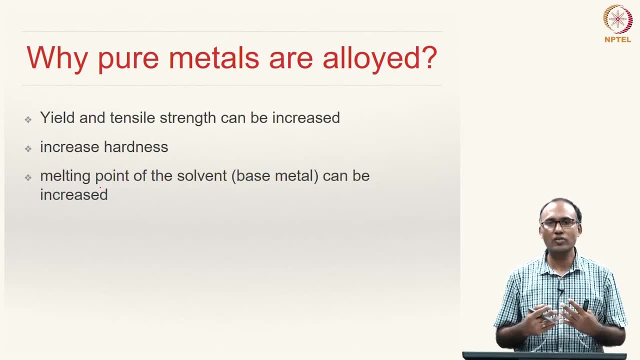 guest. So if you want to increase the melting point of this solvent, you can add some impurity or solute atoms in order to enhance the melting point of this base material, And we can also enhance the strength of the solvent at high temperatures by doing certain. 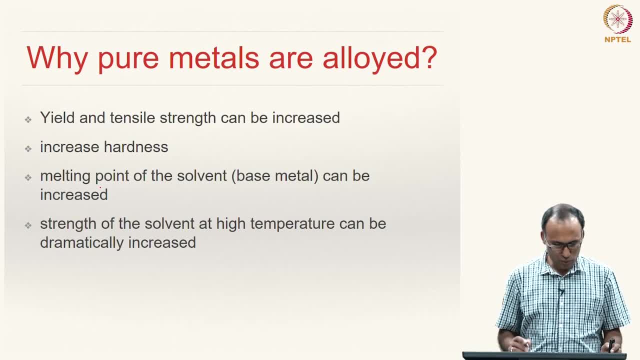 kinds of alloying. We will see such few examples doing something of that sort. And another important aspect, as we were discussing about different kinds of properties, right? So the deteriorative properties called corrosion is a deteriorative property, So that can. 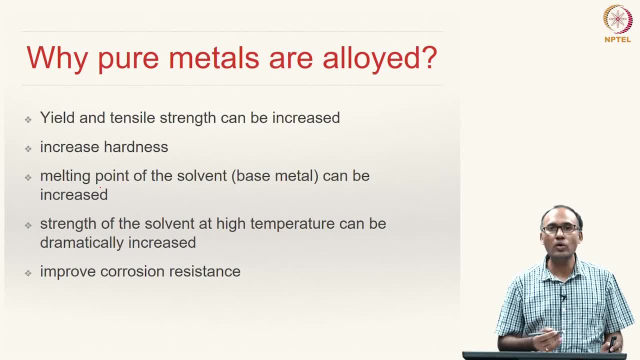 also be enhanced by alloying. So that is what we know. stainless steel is corrosion free. The stainless steel is an alloy of iron, steel and chromium and certain other materials. The resistance to corrosion is offered by elements like chromium to stainless steel, And it also enhances or improves the manufacturability. Certain materials are not cannot be manufactured. 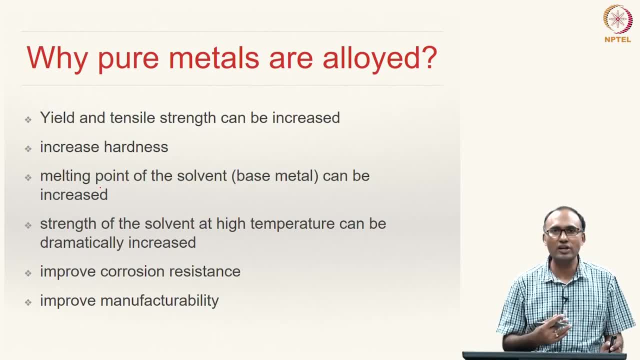 readily. certain pure metals cannot be manufactured readily And hence, in order to enhance their manufacturability, we can. we usually do some alloying So that the solvents manufacturability is enhanced by alloying it with little bit of a foreign element. And we can also sometimes 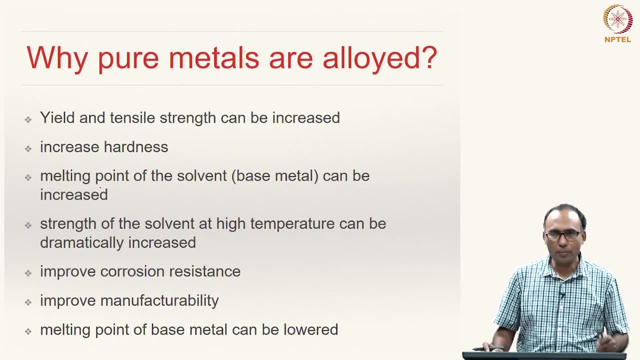 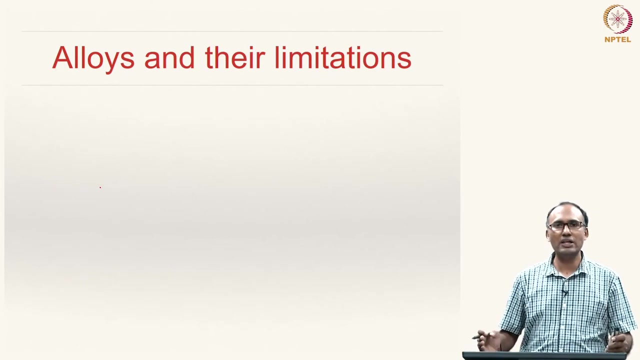 reduce the melting point of the base metal by alloying. So these are all the different advantages that one would get by alloying And hence we see alloys being more prevalent in our daily life than pure metals in their pure form. So we have- we know that there are several advantages of alloys over pure metals. Have 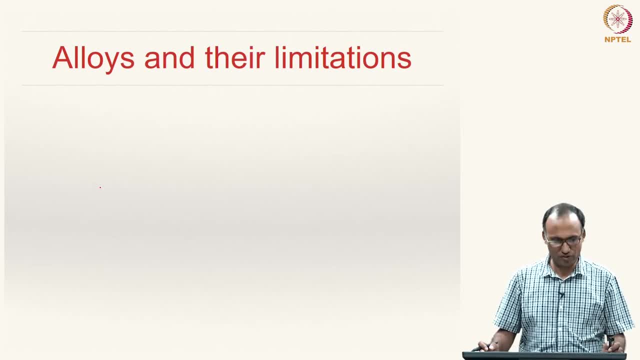 you looked at the advantages. we also need to see. are there any limitations? The limitation is that there is a limit on how much of solute can go into solution. That means you cannot add as much amount of the solute to the solvent. that is the solution. there is a limit of solubility.